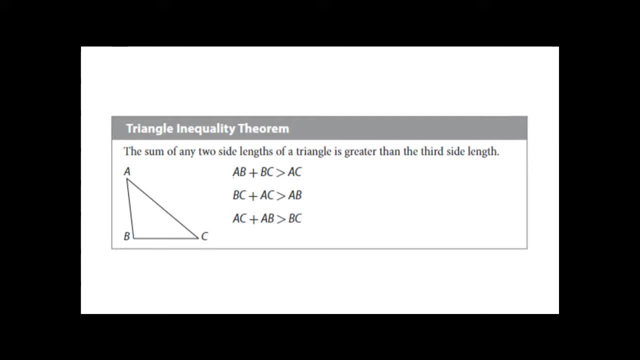 side length. so we took AB- okay, this guy right here- and we add them to BC and those two lengths, when added together, have to be greater than the total length of AC. all right, the hypotenuse, all right, and it goes the same way with all the 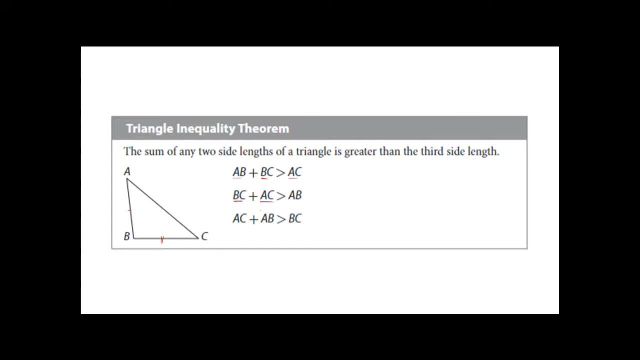 other sides. if you add up BC, this time with the hypotenuse AC, well, it's still going to be greater than the third side. all right, same thing with the hypotenuse with a, B, it'll still be greater than the third side. so it doesn't matter what order or which sides you're adding up. 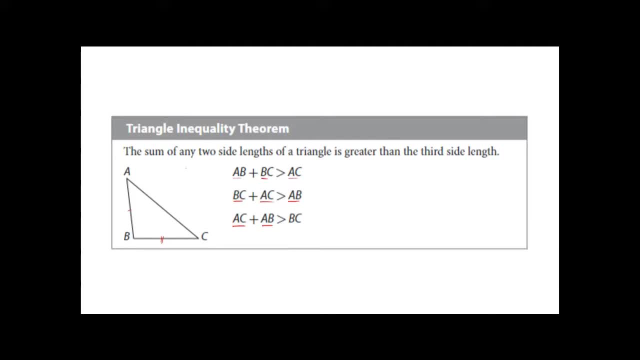 whatever two sides are adding up, okay. whichever two of the three that you're adding up still has to be greater than that third side. always okay if it's off, or one of them it's. if it's not true for one scenario, then no, it's, it's not going. 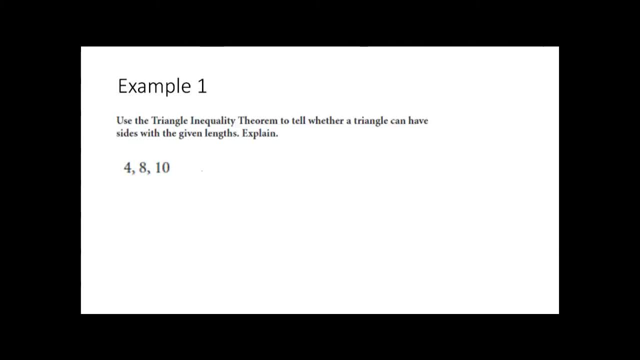 to be basically a triangle, all right. so an example one: we're using the triangle inequality theorem and we're telling whether this triangle can have sides with the given lengths. so we've got four, we got eight and ten. so let's look at our examples. we got four plus eight, and that has to be greater than our third. 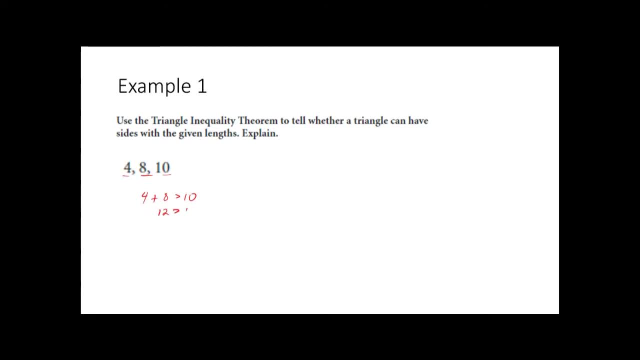 side length, which is, which is ten, and I got twelve- is greater than ten. so that's true. that checks out. but now let's think of our other situations we have. you're going to have a triangle, and you're going to have a triangle and you're. 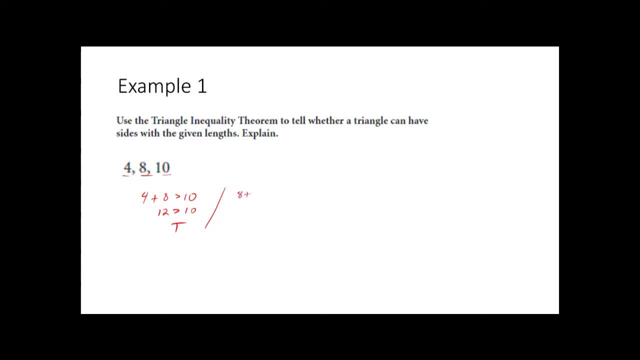 going to have eight plus ten. right has to be greater than four, and that's definitely true. okay, that checks out. and then our last combination, which is the four and the ten, which have to be greater than our third side, which is the length of eight, and fourteen is definitely greater than eight. so, yeah, 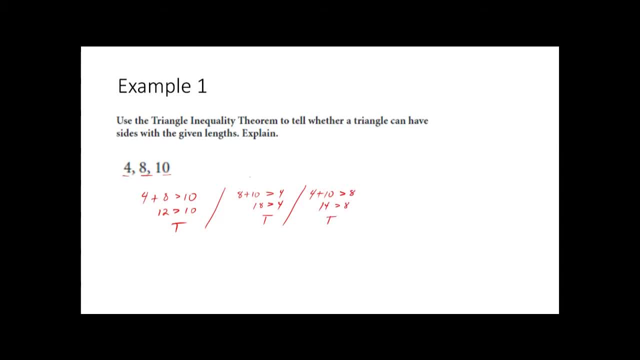 yeah, totally yeah that this, that's this triangle, can have a triangle which is greater than the length of eight and fourteen is going to have these three measurements. all right, because it does follow, follow the triangle inequality theorem, because all your inequalities are true and there you go, all right. so example two: same type of situation: we have these three. 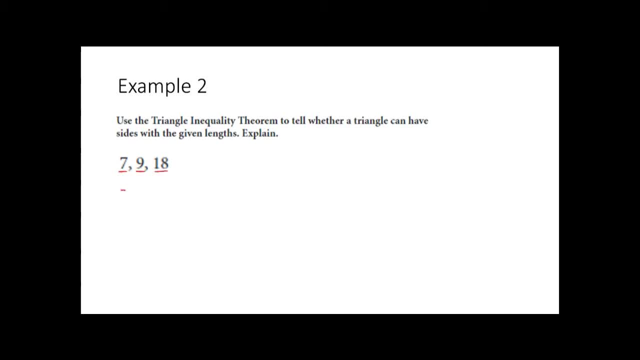 measurements. let's see if those measurements are actually physically possible. we got seven and nine, and that has to be greater than 18. and then we come across whoa, 16 is not greater than 18. that is false. so, no, no, these lengths will not work, do? 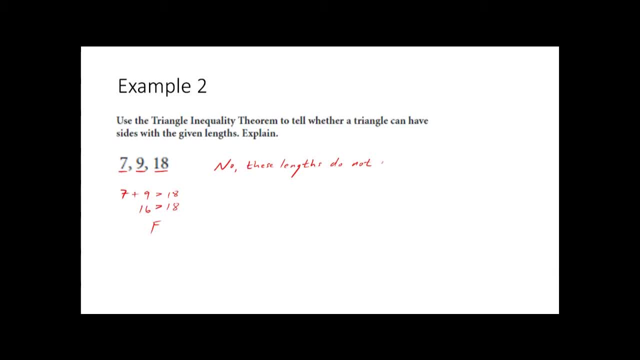 not work? and again it's because of this: 16 is not greater than 18, it's false. and again it's because of this: 16 is not greater than 18, it's false. and again it's okay. now I know you're like: what about the other measurements? well, it only takes. 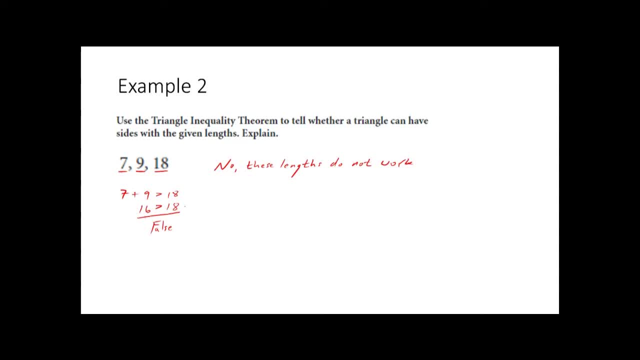 one scenario where it doesn't quite work. so one false situation. it won't work. okay, all right, your turn number one, so determine if the triangle can be formed with the given side lengths and explain your answer. so we have 12 units and 12 units of measure, and if your values are problems, I'll let you know. okay, so that takes one scenario. 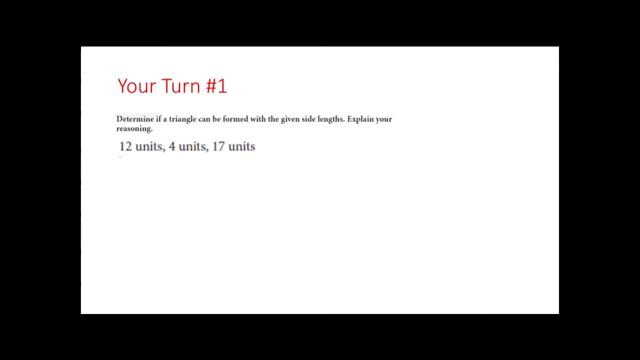 It only takes one scenario where it doesn't quite work, One false situation. it won't work. okay, All right, your turn number one. so determine if the triangle can be formed with the given side lengths and explain your answer. We have 12 units, 4 units and 17 units. 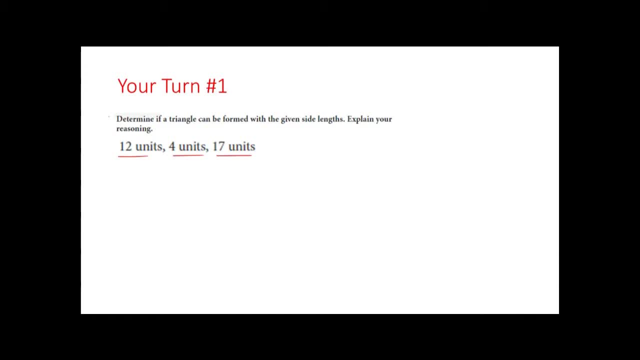 So it's just like the last two examples, okay. So see if those will work. All right, your turn. number two: same situation, just three different measurements in centimeters. See if these measurements will actually work for constructing a triangle, All right. finding possible side lengths in a triangle. 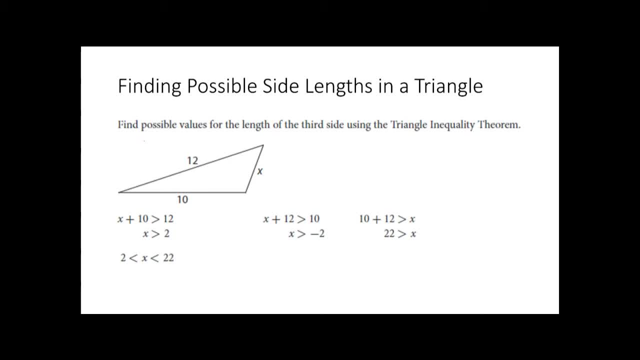 So this is a situation where we talk about what could be the range of values for our missing leg. So we know, based off triangle inequality, that 10 plus x has to be greater than our third side, which is 12.. So that's what we're setting up here. 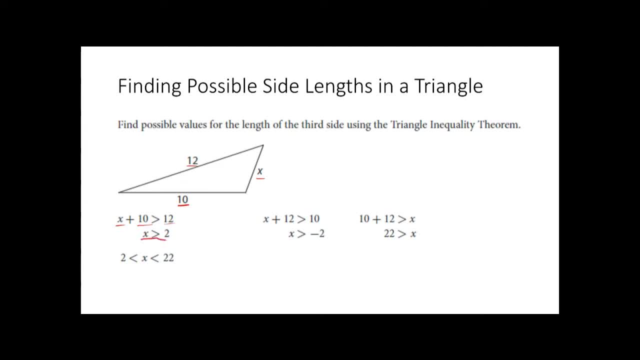 So if you actually solve for this, x has to be greater than 2.. All right, that's good to know, but what about less than Well? If we try, x plus 12 has to be greater than 10,. well, x has to be greater than negative 2,. 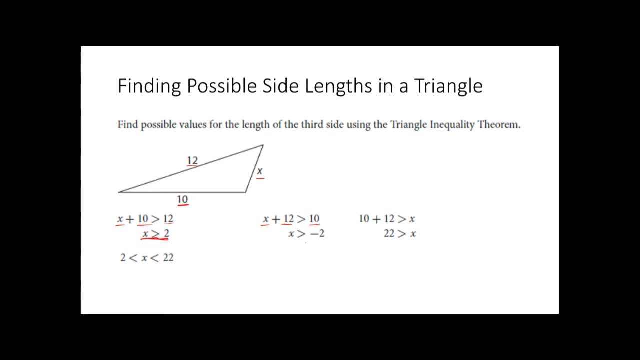 but negative doesn't really necessarily work for distance, so that's not really helpful. okay, because the integer okay. But now if you look at the other situation, you have 10 and 12, the other two sides. well, they have to be greater than our side. 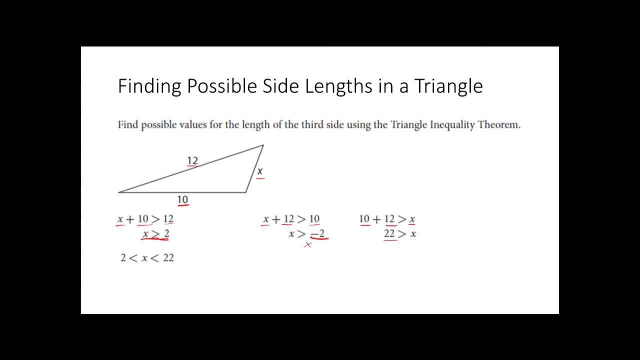 that we don't know of which is x. and then we get this: x has to be less than 22,. okay, I'm using the symmetric property real quick. It's right there for how I'm saying it. So now we have this range, okay. 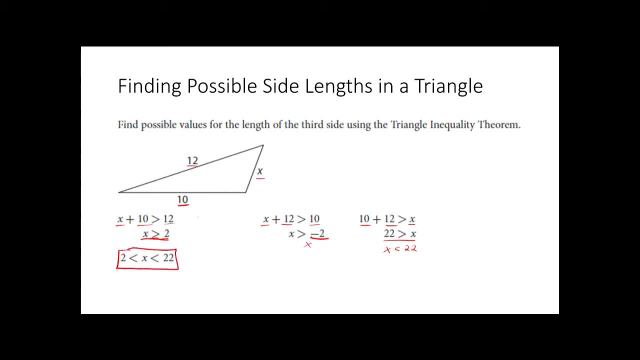 x is greater than 2, or it's less than 22.. So basically, your measurements that are possible are here, okay, So anywhere in there you can build the triangle. If it's out of that range, it's not going to work, okay. 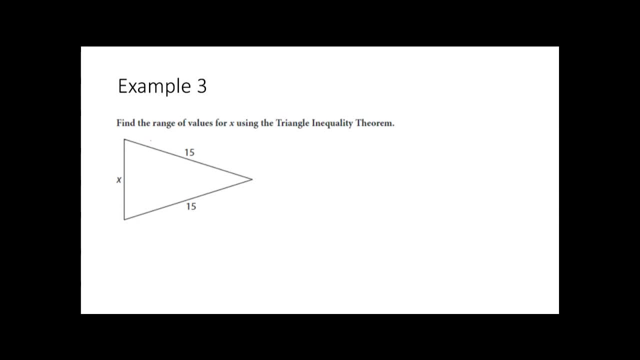 You won't be able to build that triangle, All right. so example 3,: find the range All righty then. Well, let's see We have x plus 15, and we all know that it has to be greater than the third side. 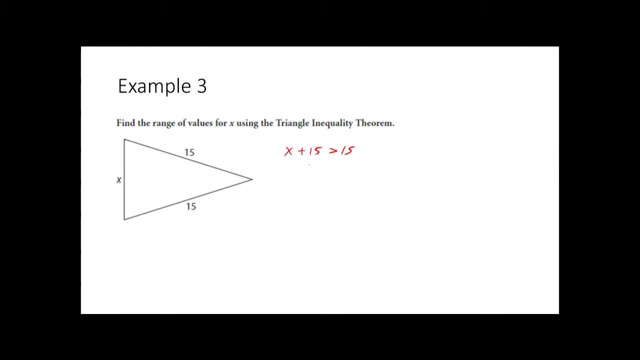 which is the other 15.. We're going to use a subtraction property- good old algebra- and we're going to have x is greater than 0. Sweet, All right, but that's only one part of it. Now we have another part. 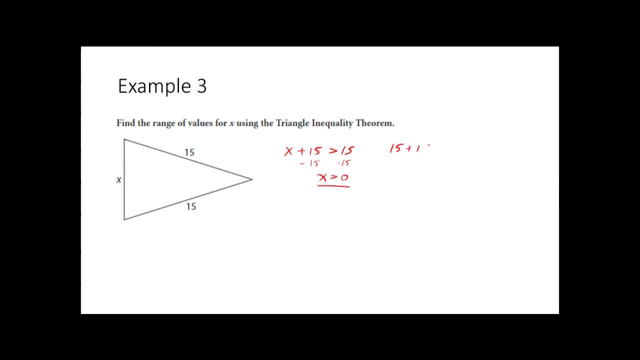 It's basically the 15 plus the other 15 has to be greater than x combined like terms. Let me apply the symmetric property real quick: x has to be less than 30, so we get this. We get: x is greater than 0, but it's less than 30.. 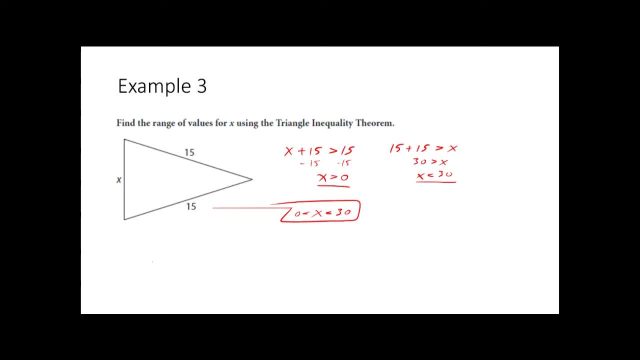 So that is going to be my range of values that I can get. okay, If I go beyond that, if I go beyond 30, if I go to 35, it's not going to work. It's not going to work. 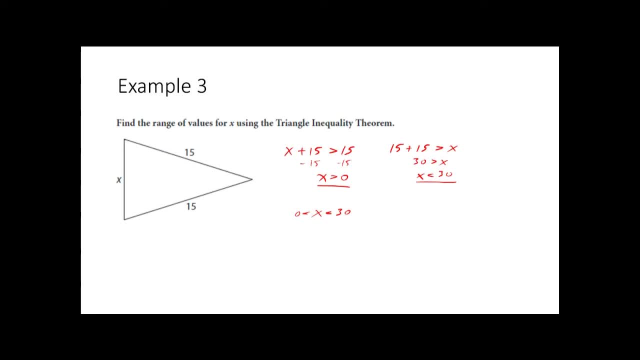 It's not going to work. I'm not going to be able to build a triangle with that length. Good to know, especially in construction: if you're ever like, hey, I need a triangular beam construction built, and then your coworker's like, hey, I made this cut. 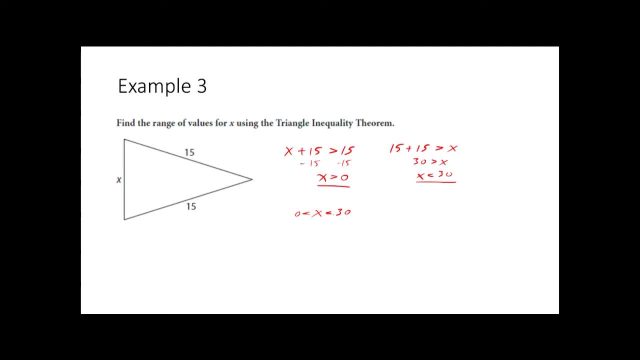 and you're like: wait, that's 35 feet, man, It's not going to work, It's a triangle, All right. so that's the real-world situation. Otherwise, you got to start building. You have your 15 bar here and your 15 bar here.